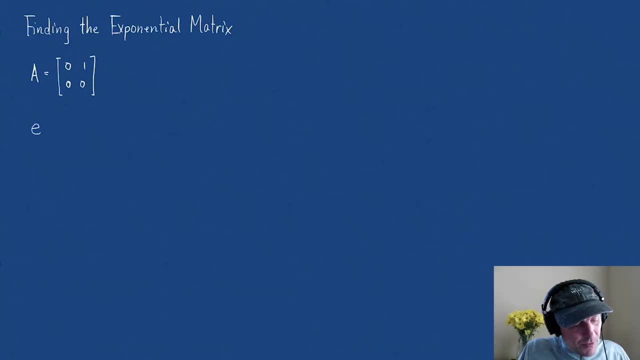 exponential matrix. So remember what this means. So the exponential matrix E to the A T, this means I plus A times T, plus 1 half A squared, T squared plus. let's go one more: 1 sixth: A cubed, T cubed. 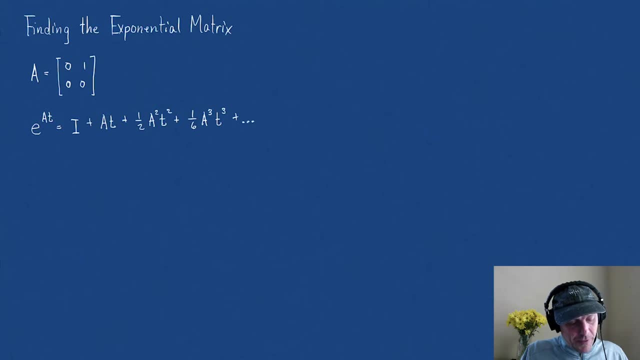 plus dot dot dot. Well, that means notice that by this third term we are going to need to find A squared, and then the fourth term we're going to need A cubed. Let's try this again. Let's try this again. 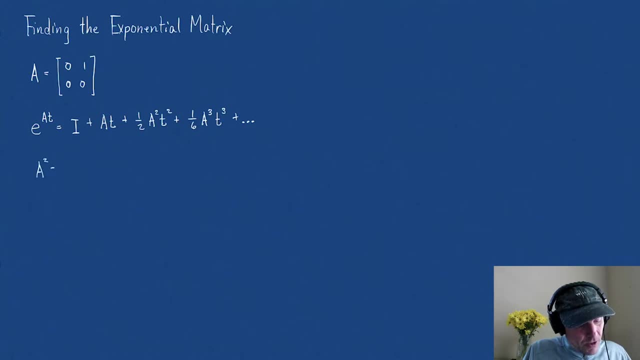 Let's try that. So let's find what A squared is. So A squared is 0, 0, 1, 0 times 0, 0, 1, 0.. Notice, that's just. oh, that's a 0.. Row 1, column 2, is 0, and row 2, column 1, is 0,. and whoa, that's. 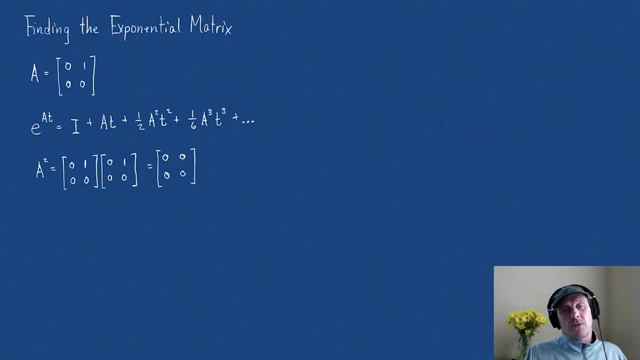 1, 0, 1.. All right, here is the matrix of 0s, and A cubed is also going to be, and so on. So when we write this, we can say E to the A. T is equal to the identity, which is 1, 0, 0, 1,. 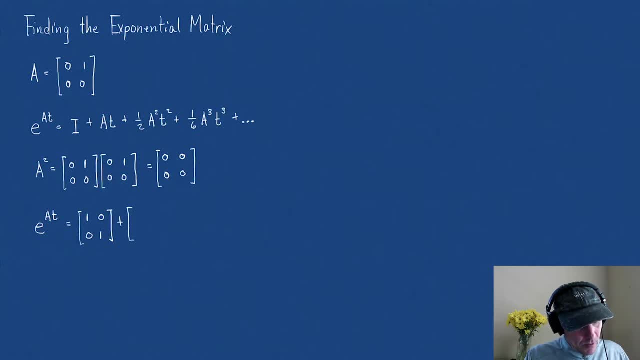 plus the matrix of A times T, That's going to be 0, 0, T 0.. So that is going to be the matrix of T. That's going to be the matrix of A T: 0, 1, 0x, 1, 0, 0, 0.. So for the Z axis, what color is the X axis? 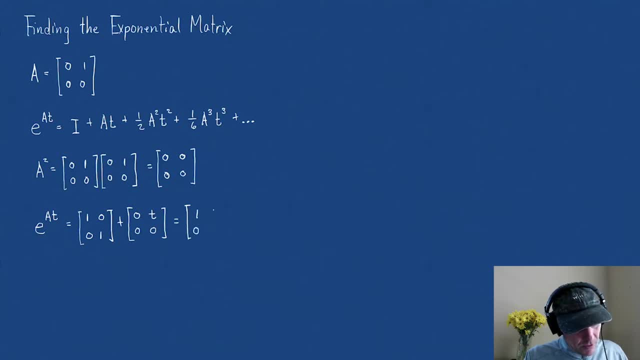 matrix of 1,, 0, t, 1,. okay, All right. now let's think about the solution that this provides us. Remember what we said. we said: if y prime equals a times y, then our solution. so then, 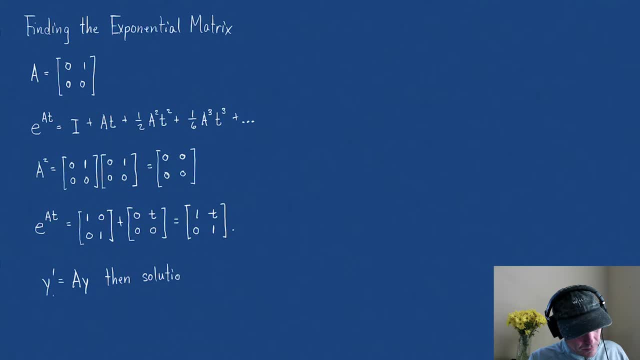 the solution is: y equals e to the a, t times. some initial conditions: y of 0,. but let's think about if we were to write this: this is y vector, remember that's y1 and y2, equals 1,, 0, t, 1, times, and let's just say our initial conditions. we don't know, maybe it's. 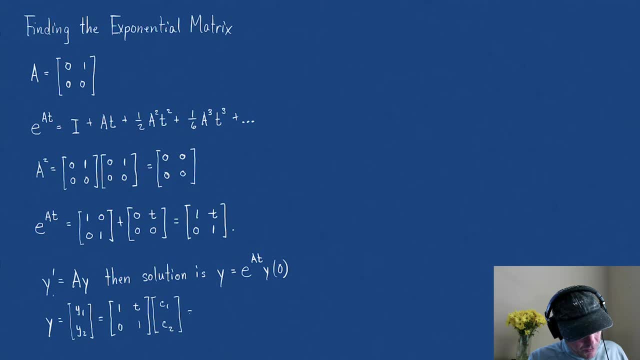 some c1 and c2,. well, if you multiply this out, this is c1 plus c2 times t, and it's also c2, c2 times just c2.. Now you might think: well, that doesn't seem that significant. well, remember what we said. 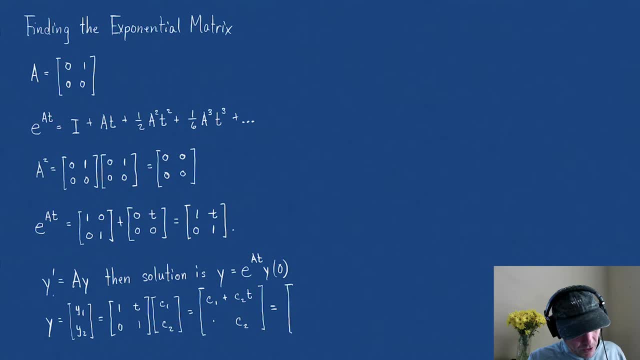 the eigenvalues were. the eigenvalues were 0, so really, this is c1 e to the 0, t plus c2 e, oops, c2 t e to the 0, t, and our second solution is c2 e to the 0, t. that is what. 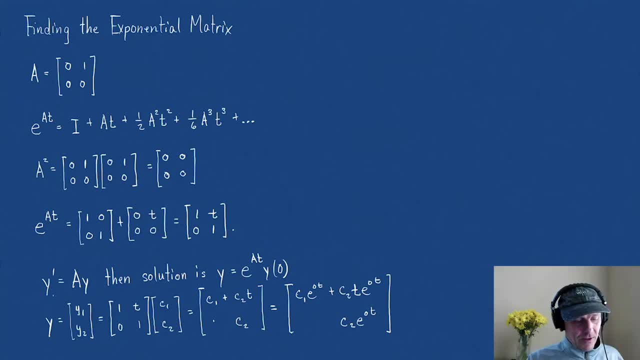 that's telling us. So it works like we might expect. All right, let's try another example. we'll start it on this one. we'll probably go on to another page rather quickly. Let's just change the matrix of a just a little bit. 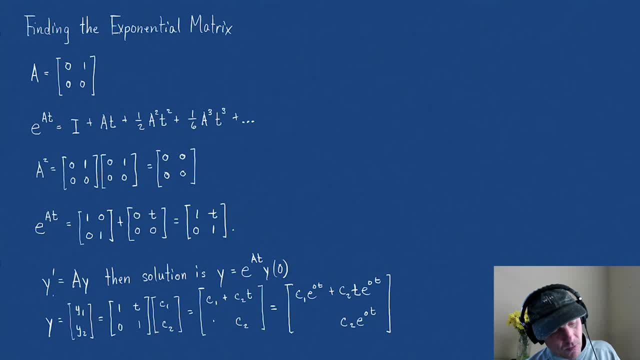 We're going to solve. solve a. oops, solve y. prime equals a. this time is 1, 1, 0, 1, times y. Now, if I was to do this with eigenvalues and eigenvectors, the difficulty here is notice. 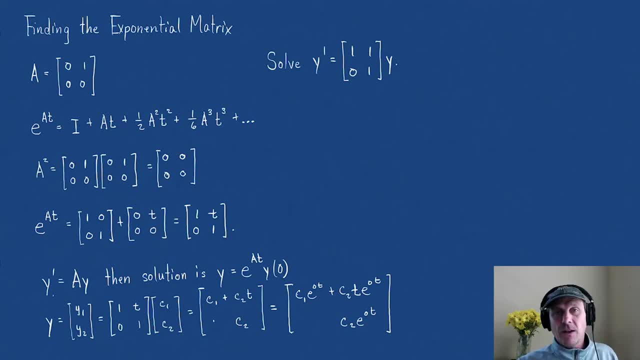 that I'm going to have repeated eigenvalues of 1 and 1, and so the problem with that, then, is I'm only going to have- I'm going to have another resonant solution, and we saw how to do that earlier. well, let's see how the matrix exponential works. so remember our 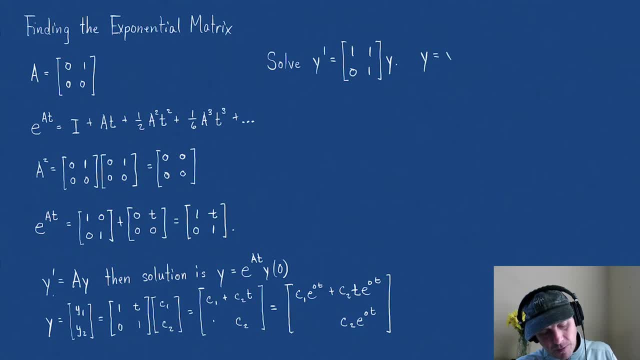 solution is of the form: y equals Some initial condition y of 0 times e to the a t. all right, well, let's just figure out what is e to the a t. well, that is, e to the a t is is i plus a, which is 1, 0, 1, 1 times. 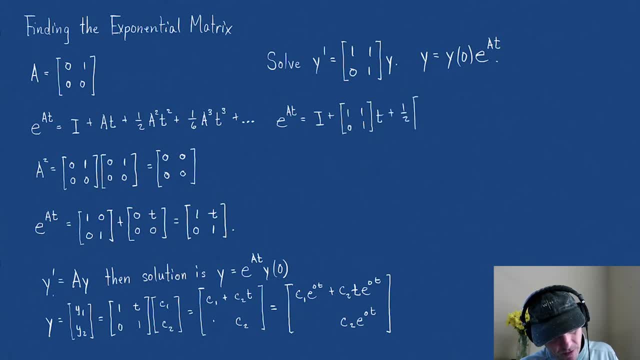 t plus 1 half times a squared. What's that? What's that? What's that? 1, 0, 1, 1 times 1, 0, 1, 1 times t squared. And we'll do one more of these, but before we do that, I'll show you what we're going. 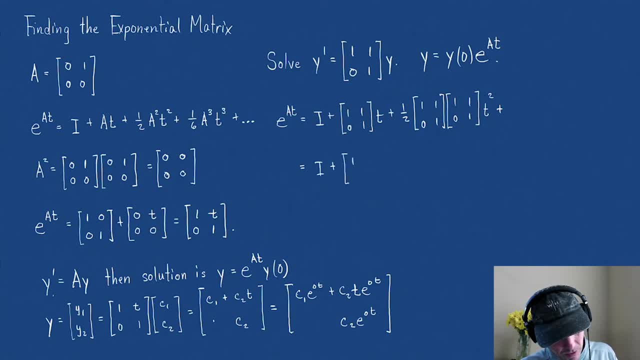 to do. We're going to go i plus 1, 0, 1, 1 times t plus 1 half times. now, if I multiply these two, I'm going to get row 1 times. column 1 is 1.. 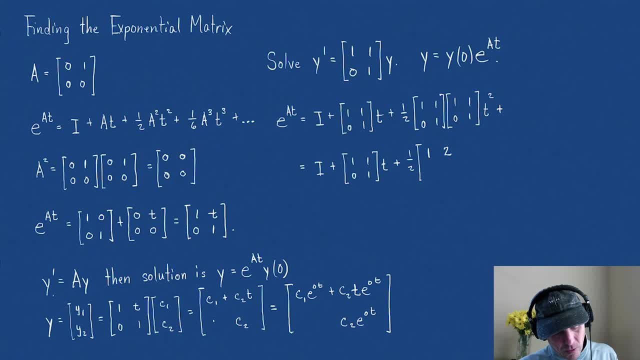 Row 1 times column 2, that's going to be a 2.. Row 2 times column 1 is going to be a 0.. And row 2 times column 2 is going to be 1, t squared plus, And what's going to happen is this: next one. 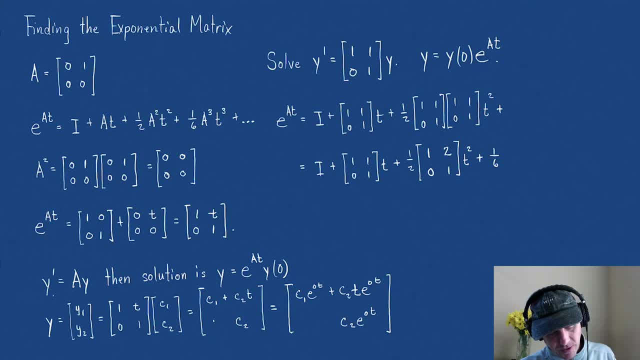 is going to become 1 over 3 factorial, which is 1, sixth times 1,, 3,, 0, 1.. It's just going to keep adding up and we have t cubed. Well, the question then becomes: how do these work out? 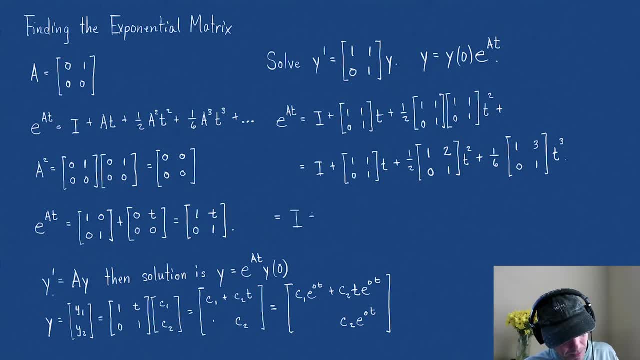 Well, let's write this out again, as i plus t, t, t 0, plus 1, half times, this is going to be a t 2t, t 0.. 0 plus 1. sixth, and I should have up here: plus dot dot dot. 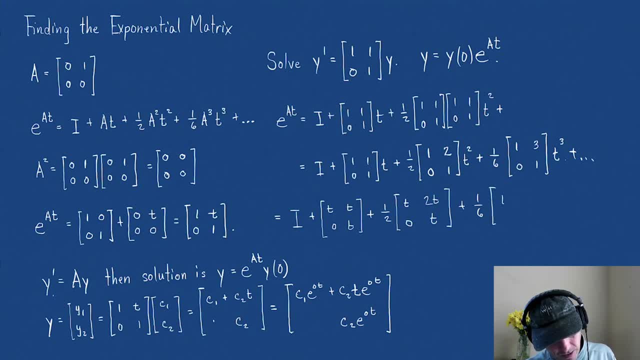 times 1, sixth times. this is going to be a t cubed, 0, 3t cubed and a t cubed, And then plus dot, dot, dot, and this is going to go on. So I'm going to take this. 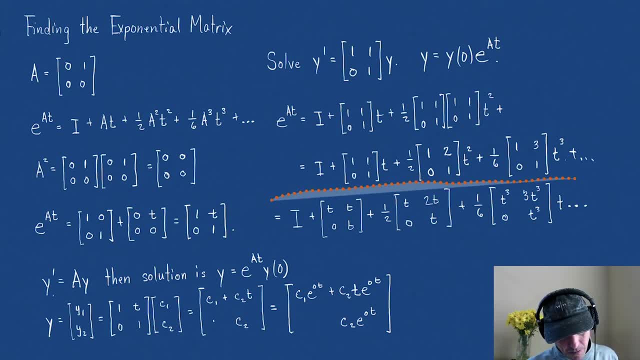 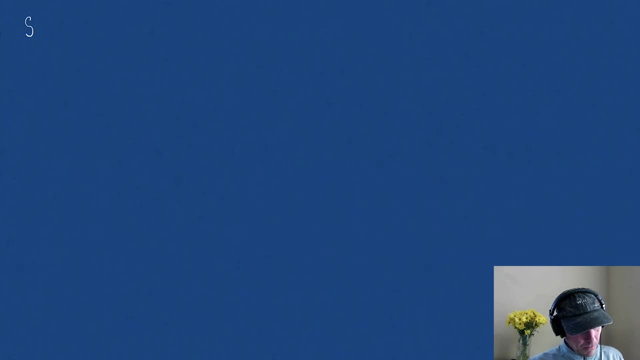 Let's go to another page. Let's see. OK, So here we are. Remember, this is, this is our e working here on e to the a t. well, let's just look at, let's just look at the one. we'll call this a 1, 1. so, in other words, if I was to just take, I'm. 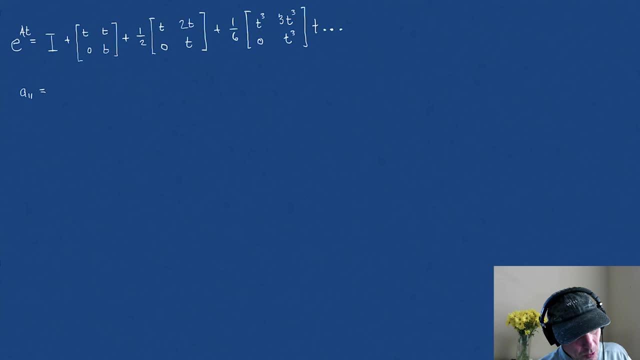 just looking at the top left component of each matrix. well, I'm going to have a 1 from the identity plus a T from the second matrix, plus a one half, and, oops, those would be T squared- T squared one half, T squared plus. then I'm gonna have 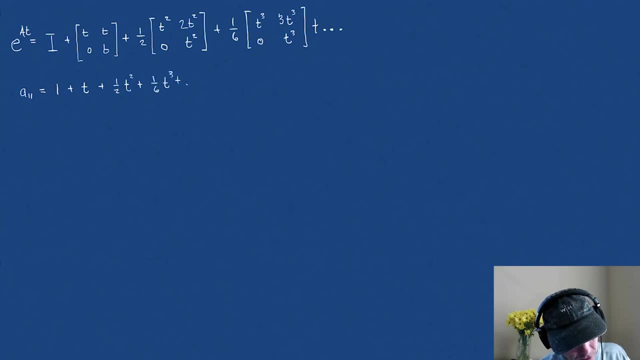 it one sixth t cubed plus. well, what we say, that is that's just e to the T, and also that's going to be the same result for a 2, 2 and this. how much we'm gonna have to get out of, out of this row of rows is gonna be: 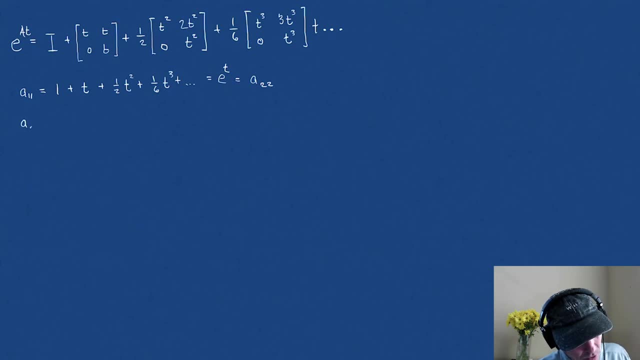 And then if we add up, let's see our a row two, column one. well, that's going to be a bunch of zeros. Then the difficult one is what in the world is a to one? Well, if we write it out, we have a zero, we have a t, then we have one half times two. 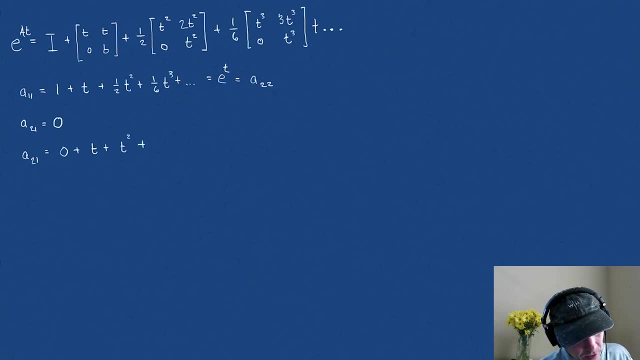 t squared, that's just a t squared plus. then I have one sixth times three t cubed. Well, that's really one half t cubed plus, and if I was to carry this out, I'd have one twenty-fourth, but I'd have a four. so that'd be one sixth t to the fourth.